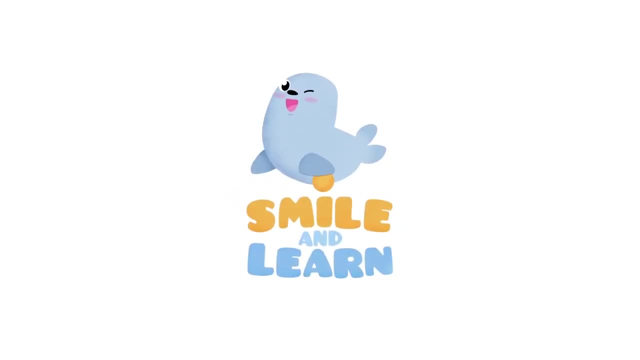 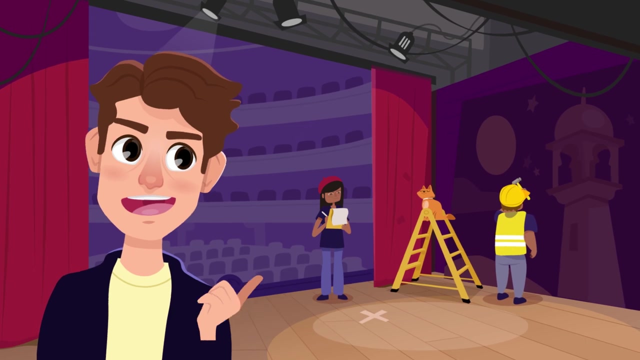 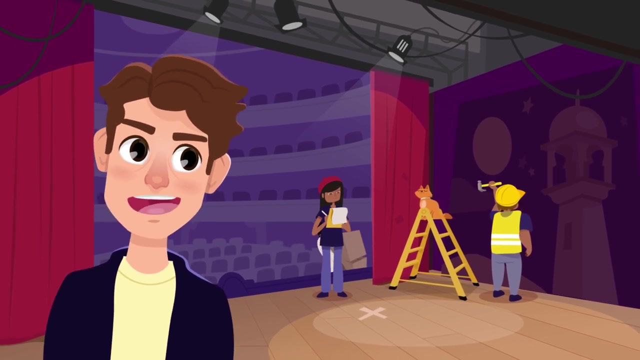 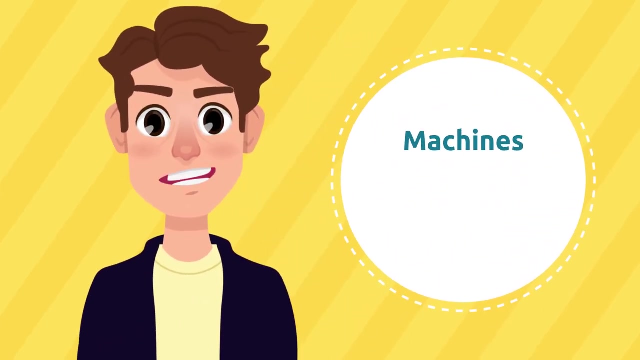 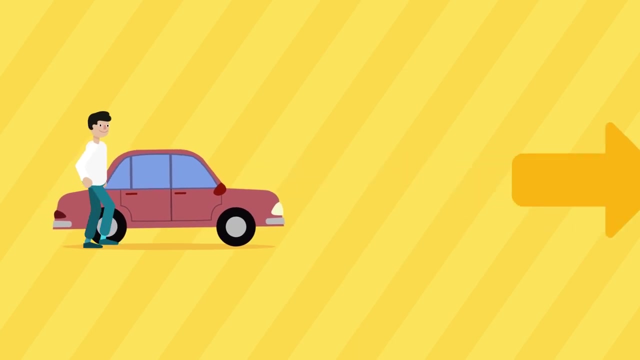 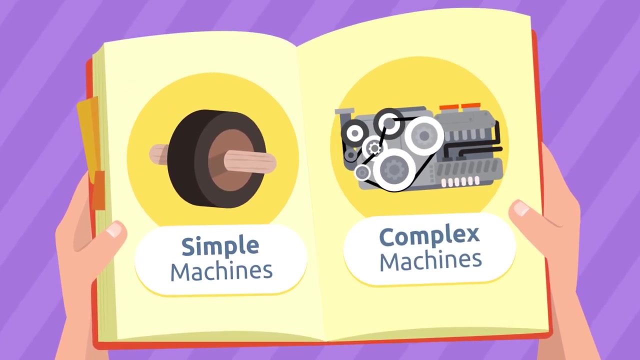 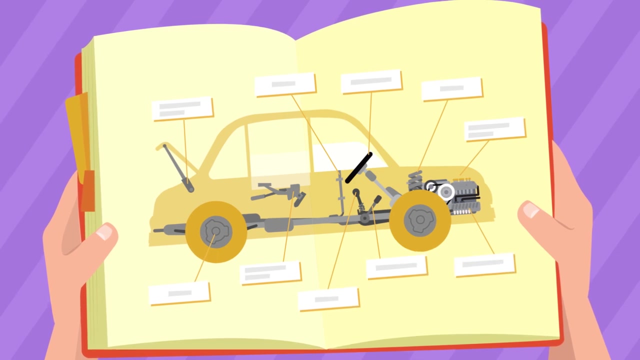 Smile and Learn. A car helps us reach different places a lot faster than walking. That's why a car is a machine. There are two types of machines: Simple machines and complex machines. Cars are complex machines because they have many, many parts. There are also simple machines that have one or fewer parts. 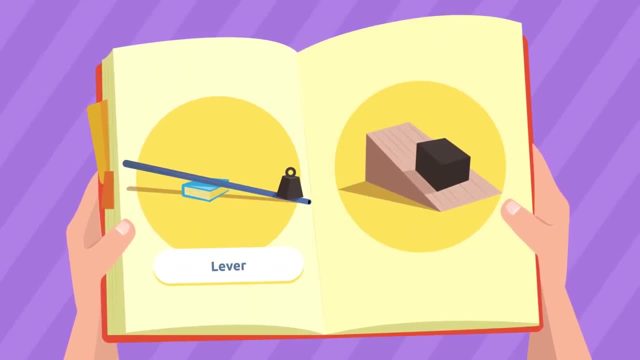 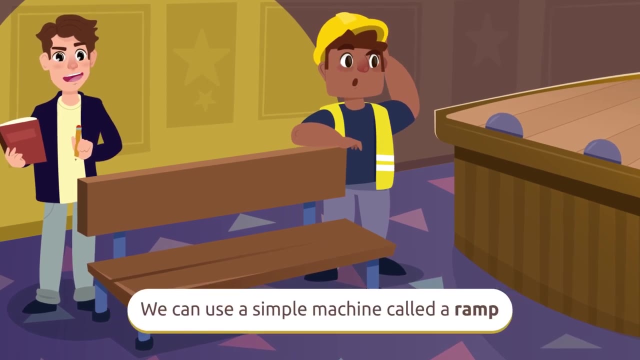 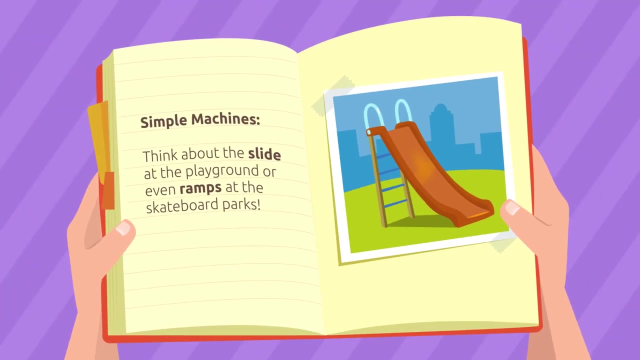 We will use simple machines today, Such as a lever and a ramp. We need to move this bench on the stage. We can use a simple machine called a ramp. I am sure you have seen them before. Think about the slide at the playground or even ramps at the skateboard parks. 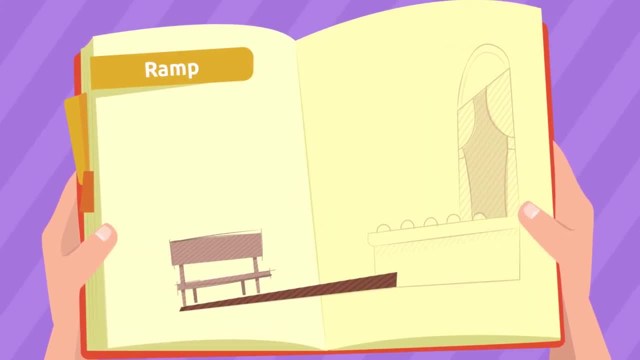 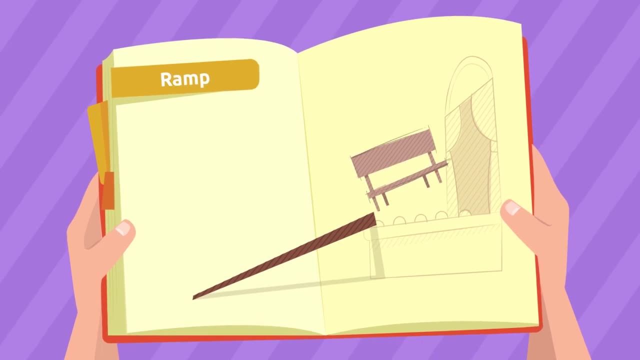 Let me show you. By placing a flat surface at an angle between the stage and the ground, we create a ramp that will easily allow us to move this bench up on the stage. Now, that was easy, It was fun. Wait, what's that under the bench? 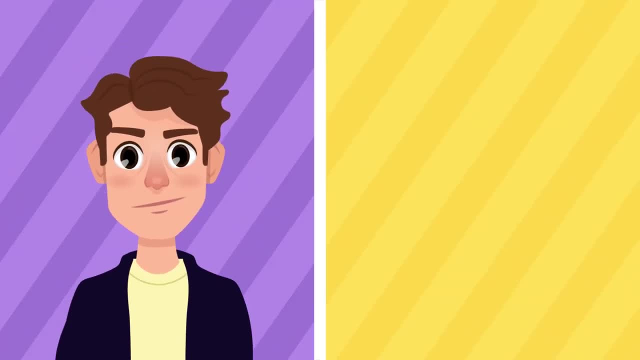 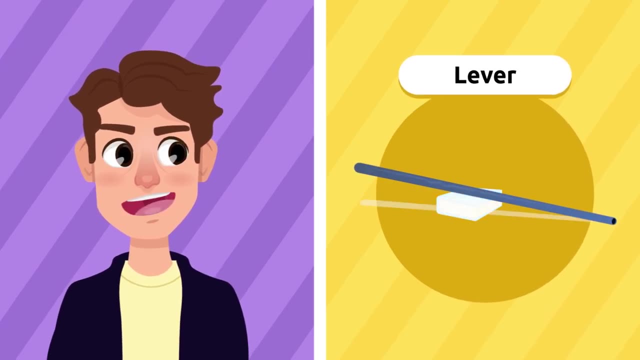 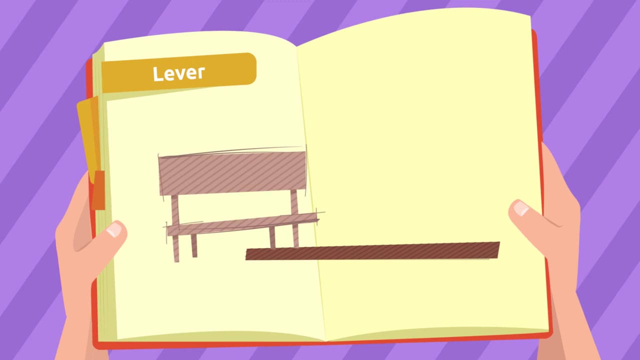 But it's too heavy to lift. Maybe we need another simple machine. Hmm, how about a lever? All we need is a stick and a book. Let's take a look. We can place one side of the stick under the bench and balance it on the book. 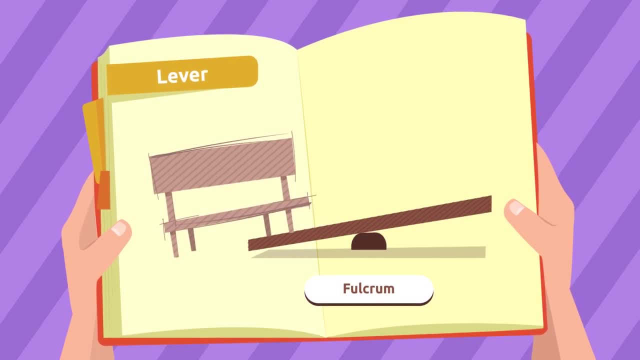 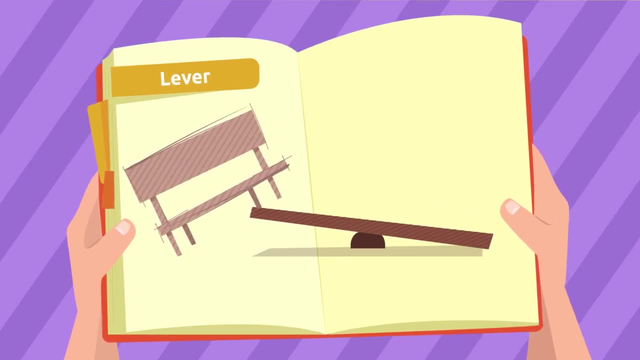 The book becomes the fulcrum, which is the support element of the lever. A lever needs to lift the object on the other end When we push on one side, kind of like a seesaw- Oh look, it's my sports sticker. 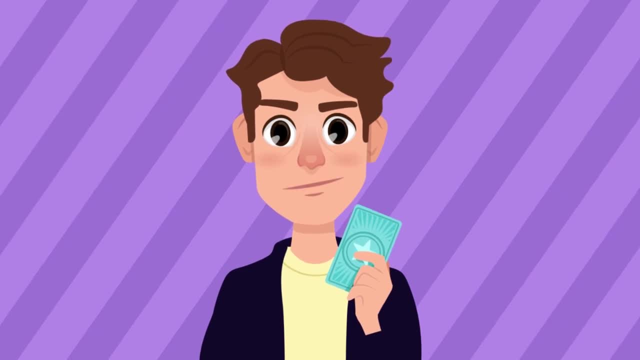 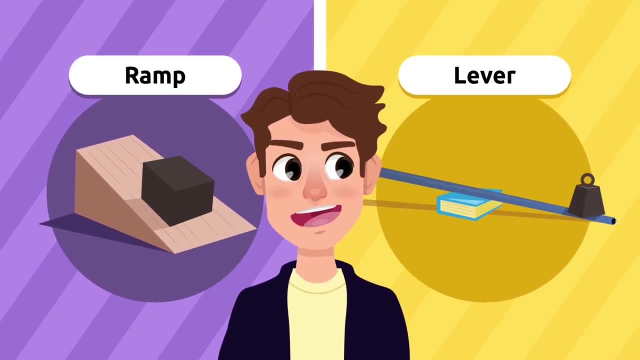 I lost it yesterday. I'm so happy we found it. Let's see: We used the ramp to move the bench up on the stage. Then we created a lever using a stick and a book to lift the heavy bench And found my missing sports sticker. 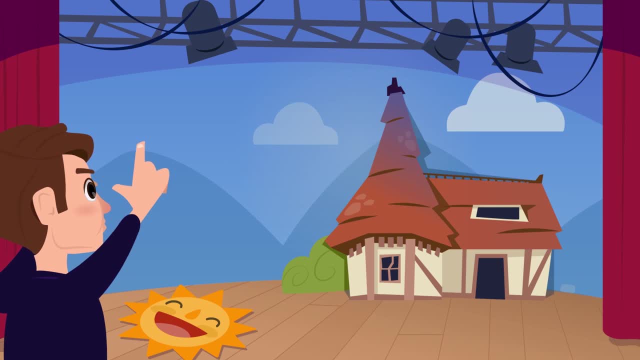 For our next task, we need to move the bench up on the stage. Then we created a lever using a stick and a book to lift the heavy bench. Then we created the lever and the stick together. For our next task, we need to move the sun to the other side of the stage. 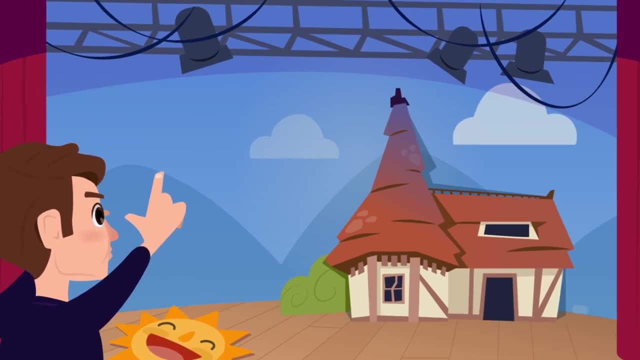 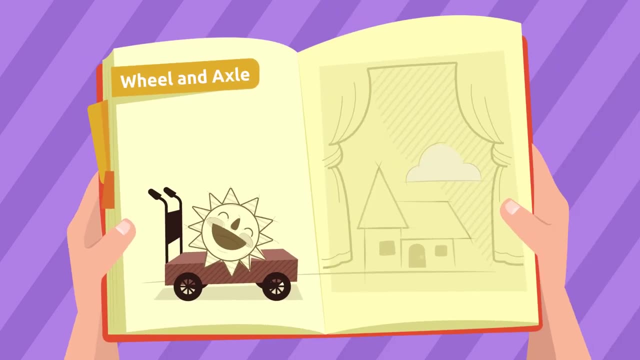 and lift it up over the house. We can use a wheel and axle and a pulley. We can use this cart Which has a wheel and axle. Let's look: When we push the cart, the wheels on this cart spin. 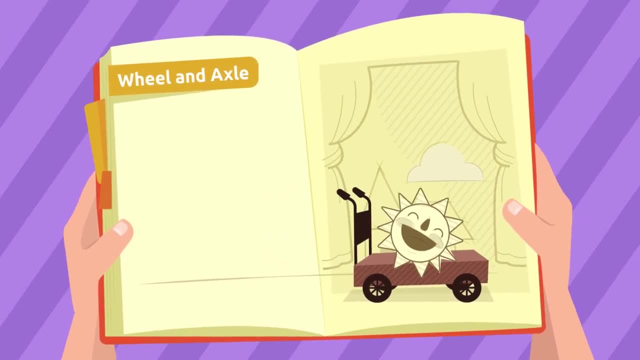 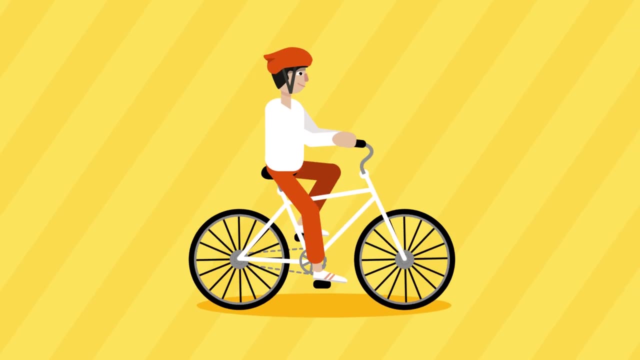 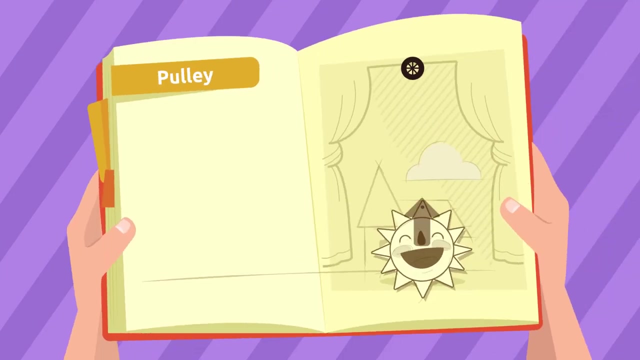 helping us move the sun across the stage. It's the same as your bike at home. So when we pedal our bike, The wheels spin to move us forward. The bike is a great example of wheel and axle in action. Now, in order to lift this sun, we can make a pulley by looping a rope around the wheel above. 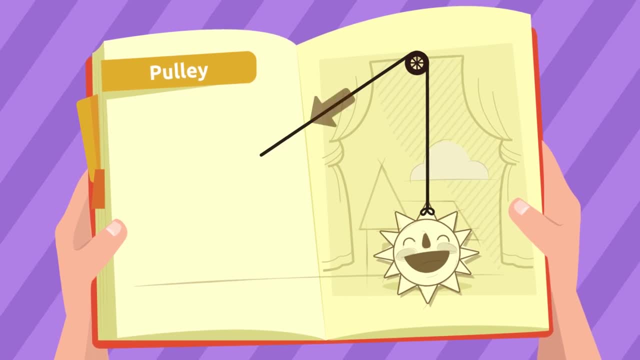 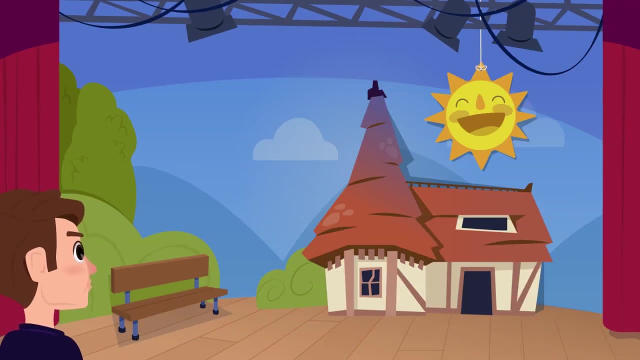 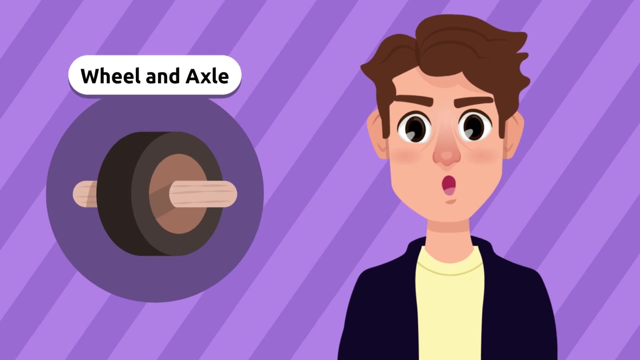 We will attach the sun on one side of the rope and pull from the other side. The pulley will help us lift the sun off the ground. Super cool, right, Let's see. We used the wheel and axle from the cart to move the sun across the stage. 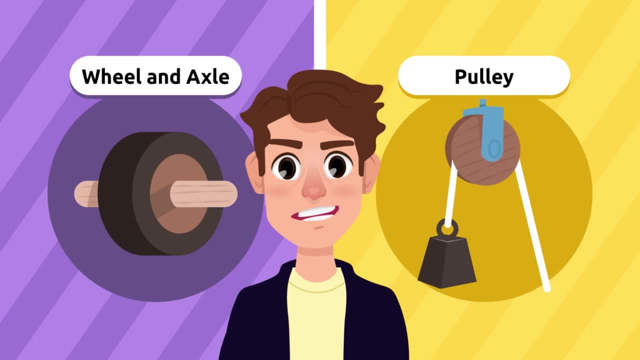 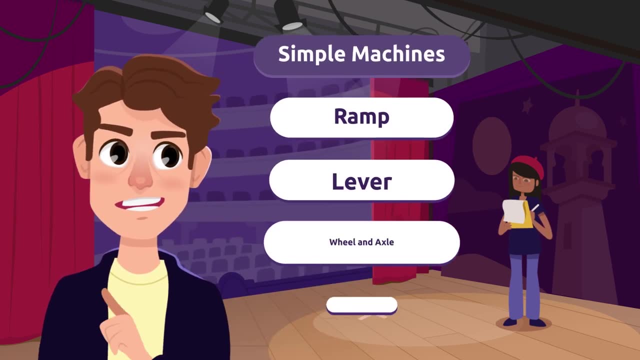 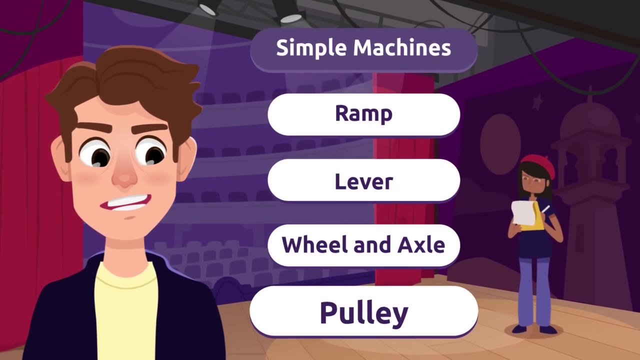 Then we created a pulley with the wheel and rope to lift the sun to its right place. We did it. These simple machines were really useful. The ramp, the lever, the wheel and axle and the pulley all helped us move and lift heavy objects, saving us time and energy. 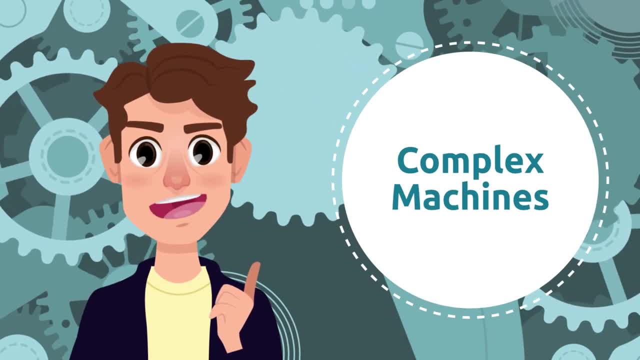 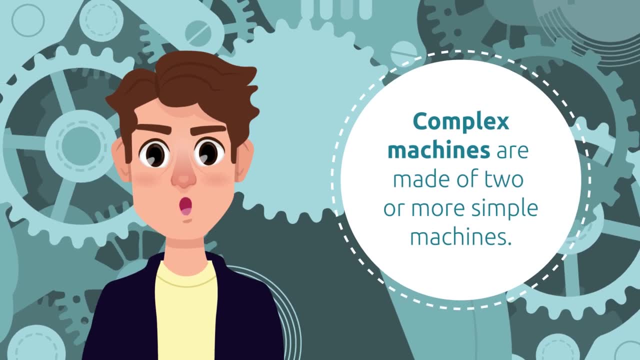 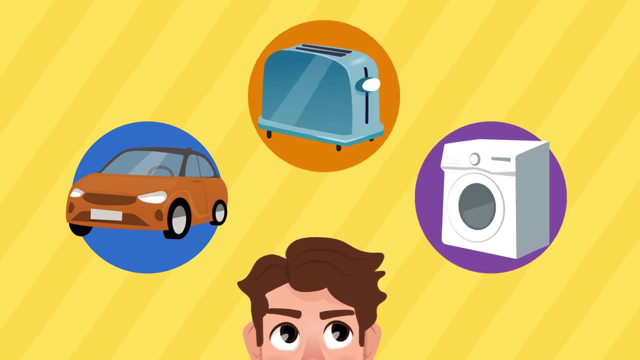 We didn't use complex machines today, but we use them all the time. Complex machines are made of two or more simple machines like the ones we saw today, Sometimes even hundreds. Cars, toasters or washing machines are examples of complex machines. 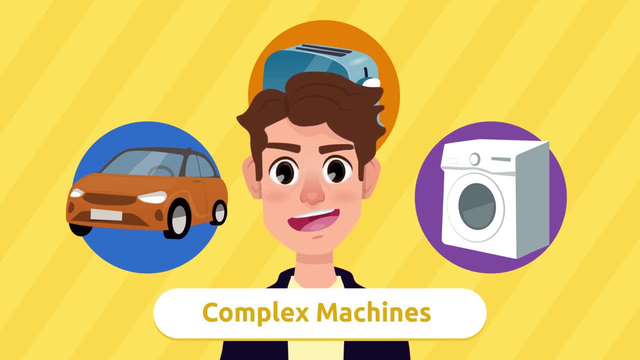 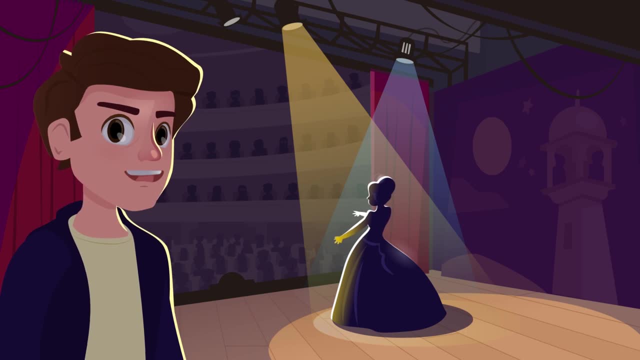 Amazing. It looks like both simple and complex machines are super useful and important in our lives. Thanks for joining me while we explored machines. Remember, simple or complex machines make our lives easier. It's showtime. I have to go Shh. 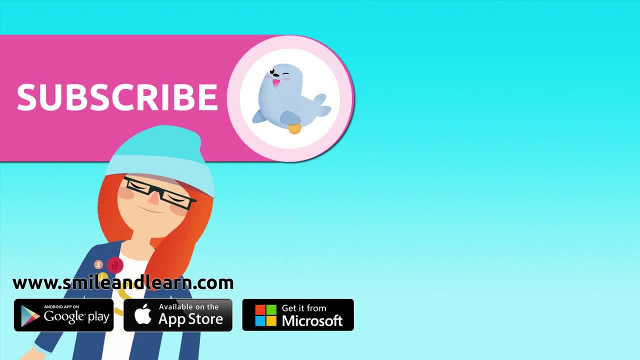 Subtitles by the Amaraorg community.